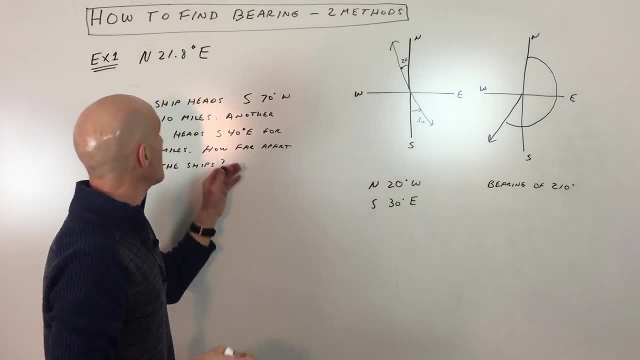 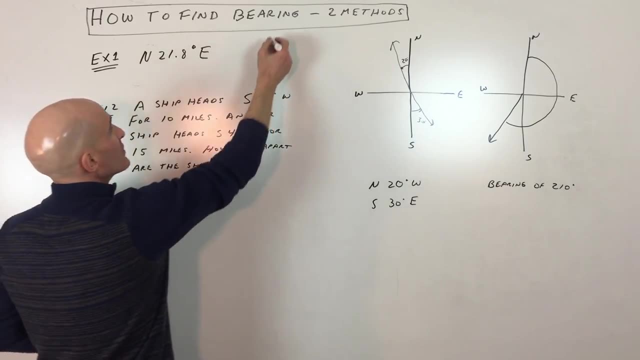 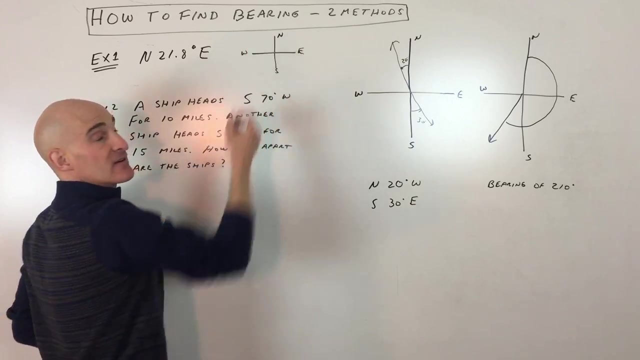 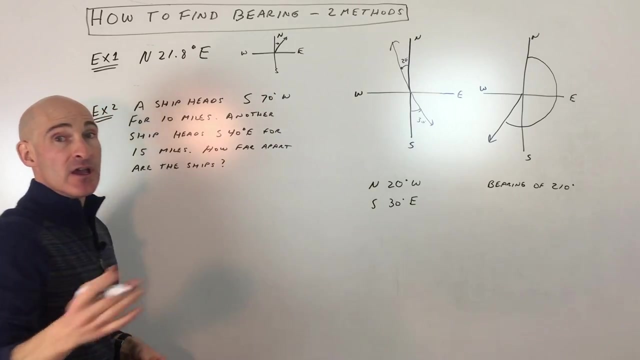 So the two different ways of measuring bearings. Let's go through a couple examples together. So it says: say you're heading at a north, 21.8 degrees east, Okay. so this one is just saying: okay, we're going to face north, We're going to head towards the east. Remember, never eat sour watermelon. You go in that direction like that. So start facing north and we're heading 21.8 degrees towards the east. So that's right there. A second example: it says a ship heads south, 70 degrees west. So you start facing north and you go 30 degrees towards the east. That's our angle, right there. 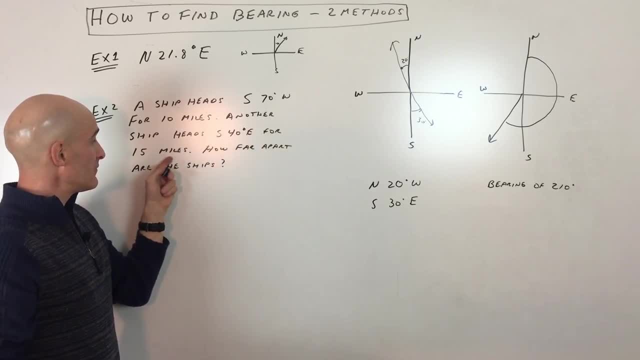 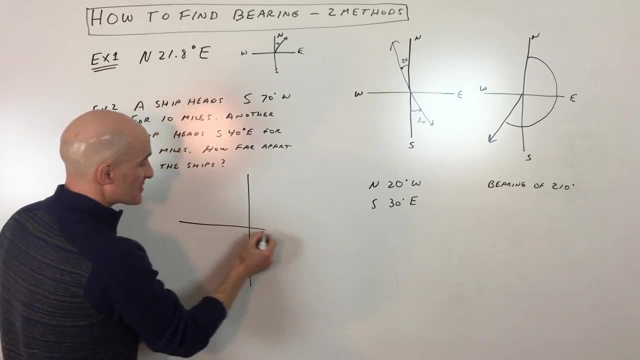 10 miles. Another ship heads south, 40 degrees east for 15 miles. How far apart are the ships? Okay, this is a good problem. Let's see if we can draw this. What you want to draw is: you want to draw your coordinate axis like this: Label your directions: north, east, south, west. Start at the origin. 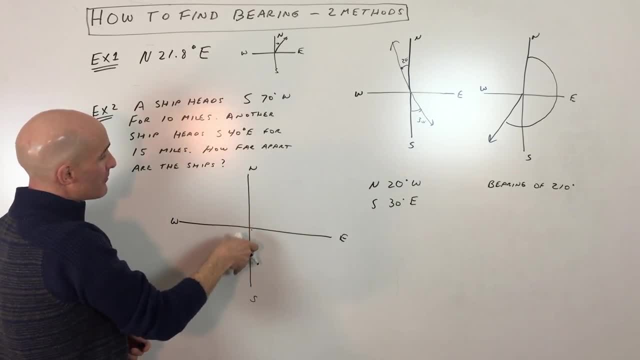 and one ship is heading south. So we face south 70 degrees towards the west, like that. So this is a 70 degree angle and it's going for 10 miles, So I'm just going to write 10 miles. The other one: 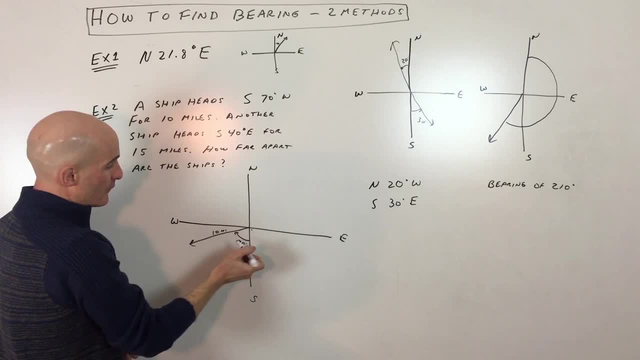 is south, 40 degrees east. So we start facing south and we head 40 degrees towards the east, approximately right there, and that's for 15 miles. It's a little bit longer. So that's south, 40 degrees towards the east. Now we're trying to find the distance between these two ships and that's 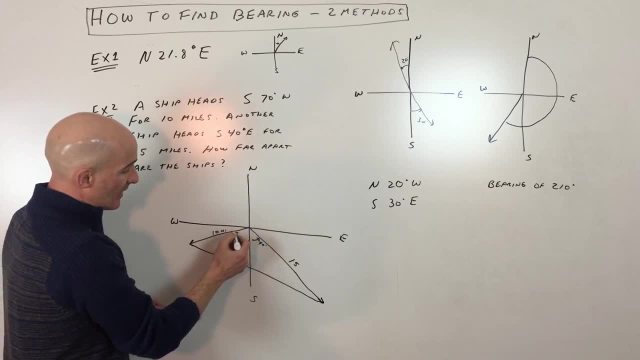 right there and what you notice is we have this side angle side situation. So when you have side angle side, like that, and you're looking for this length here, you can use the long angle side situation. So when you have side angle side, like that and you're looking for this, 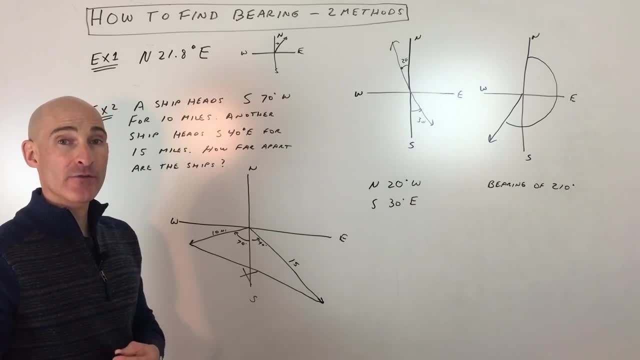 long angle side situation. So when you have side angle side like that and you're looking for this law of cosines and you can review some of my videos talking about law of cosines if you need to review that, but we'll set it up here. So basically we have a total of 110 degrees for 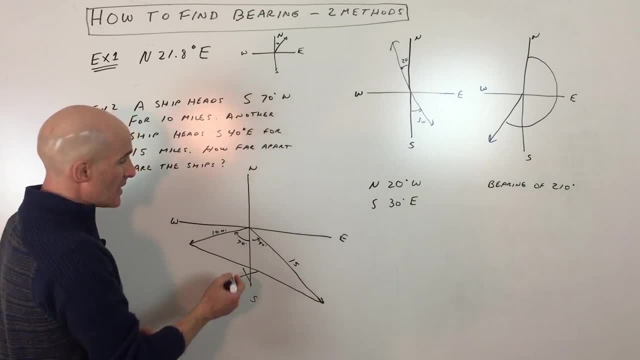 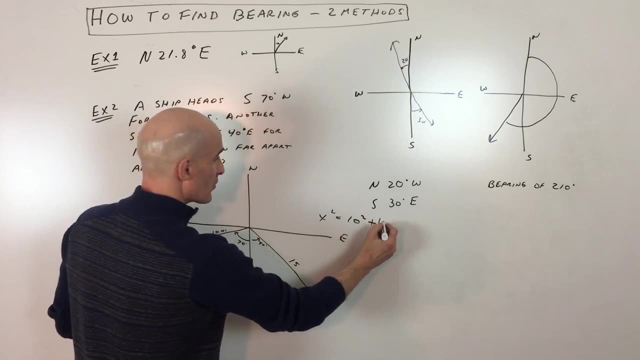 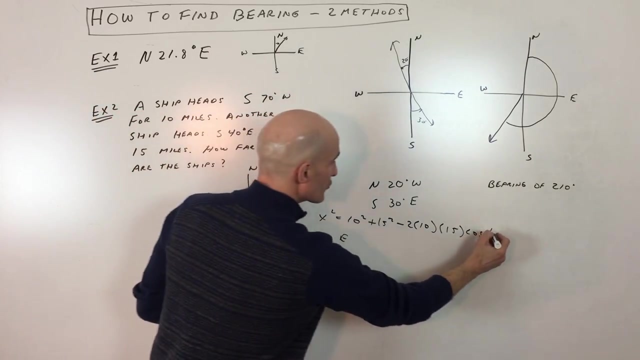 that angle, that's in between the two sides, 10 and 15.. So what we would do is we'd say: x squared equals 10 squared plus 15 squared minus 2 times 10 times 15 times the cosine of the included angle, which is 110 degrees. Then what you would do is: since you're just solving for x and